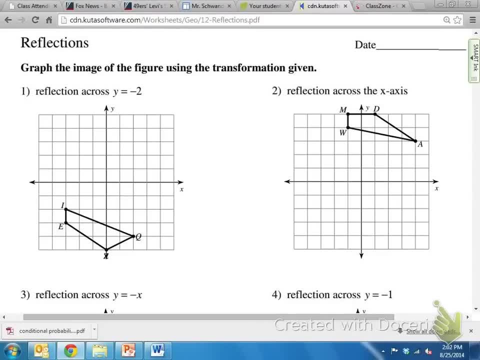 All right. so we're looking at number one here on this worksheet, and it's the directions say: reflection across y equals negative two. So we've done examples of reflecting over the x-axis and the y-axis, which are easy to find, but y equals negative two. So this line exists not on one of. 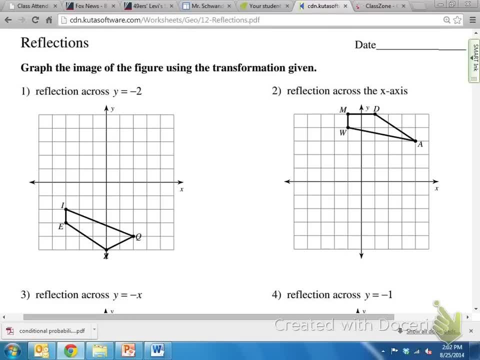 the axes, but somewhere on the graph. Here's the way I like to think about it. So it says that y is equal to negative two. So I know that it has to cross. y equals negative two. So I'm going to put a dot on y equals negative two. I know it has to cross there, but here's the thing. 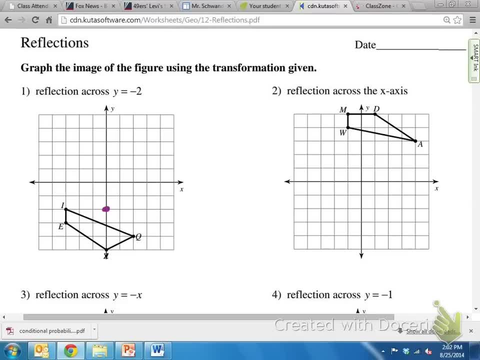 with that line. If y only equals negative two, y can't be any other number. y can't equal negative three, y can't equal negative four. y can't equal seven, because y equals negative two. So no matter what x is, x could be any number. 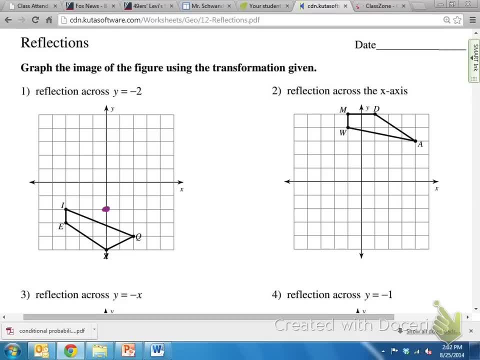 x could equal seven, x can equal five, but y will always be negative two. So when I make my line, my line can only go across: y equals negative two. So that's why I'm putting my mirror right there. So my mirror can only happen, it can only touch. y equals negative two. So that's where my mirror 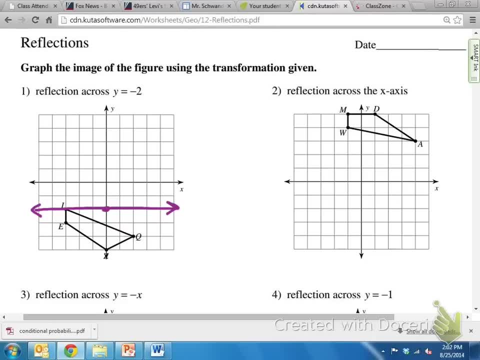 goes. Now we know where our mirror is. We go to each point and count how many units it takes to get to the mirror and then we count that many spaces. Now we go to what if past the mirror, to put the next point. So notice point. I Look at point I there. 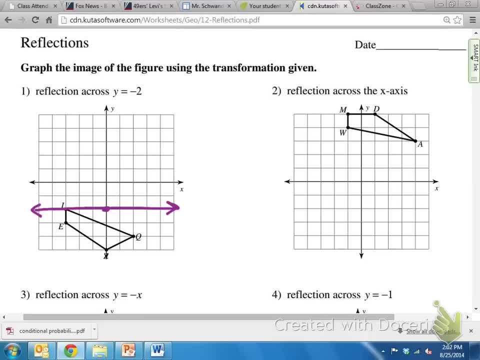 at the top left. It's on the mirror. So if my point is on the mirror I don't need to move it. It stays right where it is Done. So now we move to another point. Let's go to point E. So from point E to the. 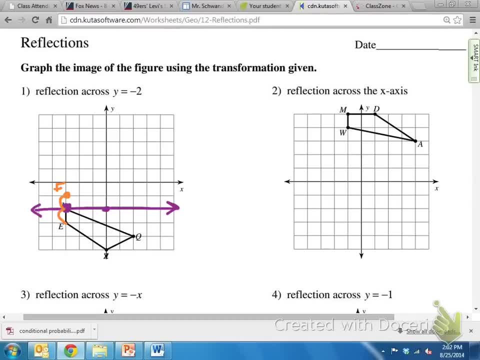 mirror. it takes one unit. So I go one unit above the mirror and that's where E prime will go. Okay, let's go to x down here towards the bottom. X takes one, two, three, four. So that's right here. So I've got. a point E and a point. Now we move to point four and it will be one unit. So if I go one unit above the mirror, that's where E prime will go. Okay, let's go to X down here towards the bottom. X takes one, two, three.